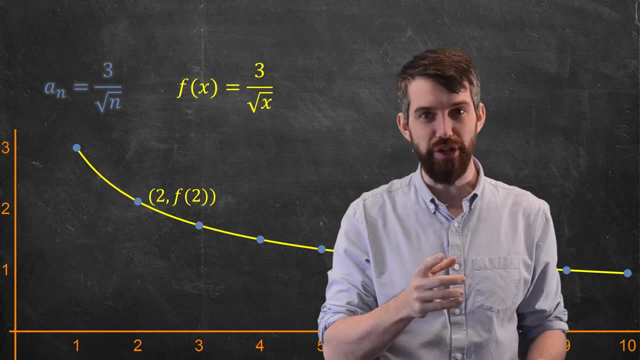 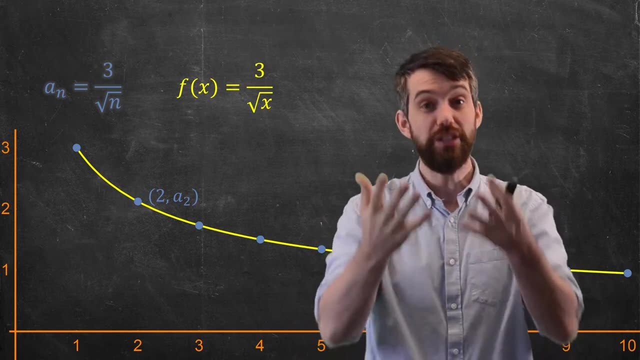 I'm talking about it through a sequence: instead of 2f, of 2,, it's 2a2.. The second term of the sequence gives me the height of a particular point and the x coordinate is given just by the 1, the 2, the 3, the value of n in general. 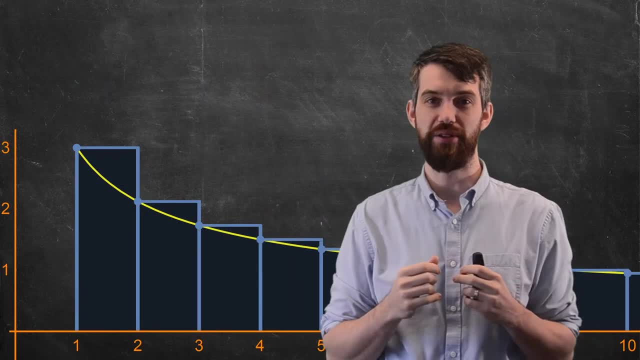 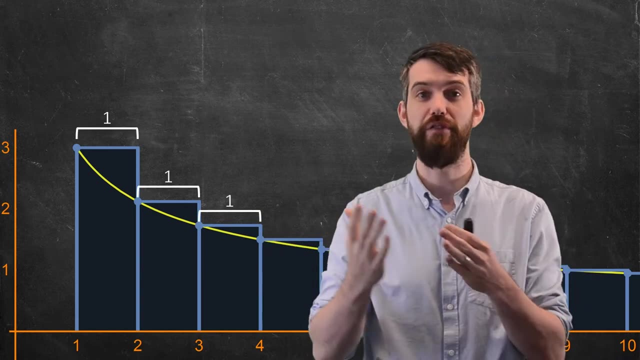 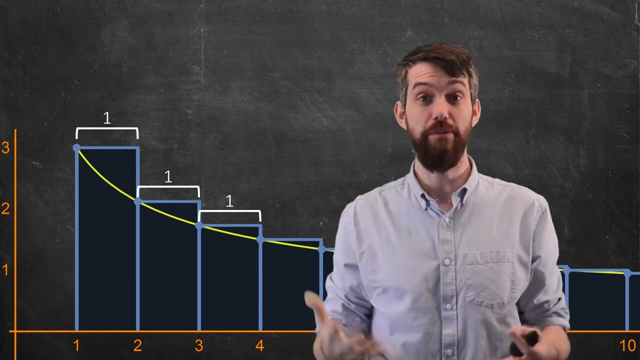 Now what I'm going to do is overlay on this graph a bunch of rectangles, And the idea for these rectangles is that the widths of them is all just going to be the values 1.. They're going from 1 to 2,, 2 to 3, and so on, But the height of these are given by the left. 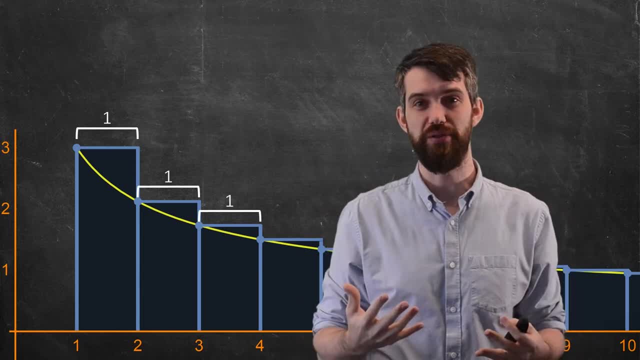 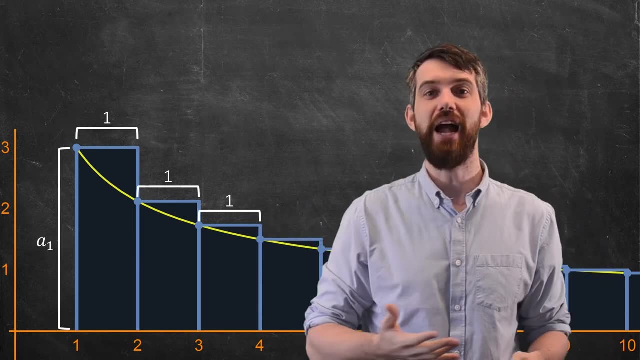 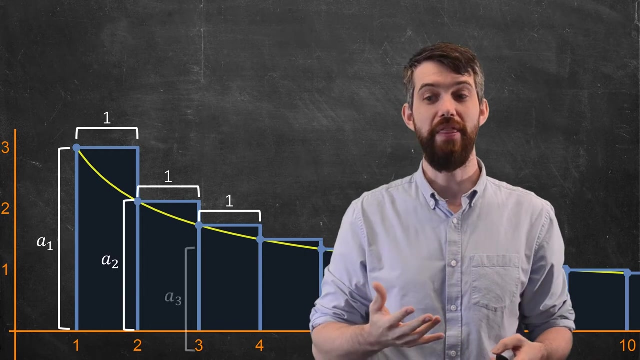 endpoints of the curve, As in they're given by the sequence values. So for the left-most rectangle, its height is going to be just a1.. For the second one, it's height is going to be the left endpoint. on the 2nd interval, the region 2 to 3.. It's going to have a height of a2.. And then it's. 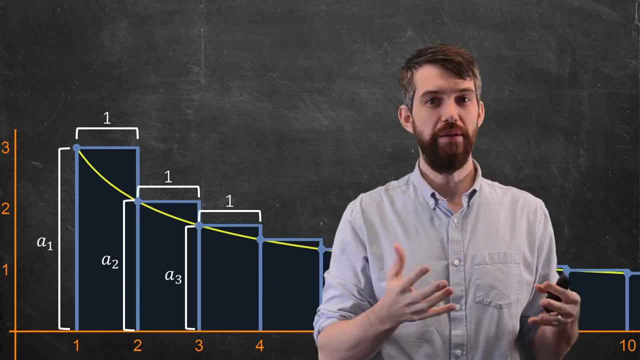 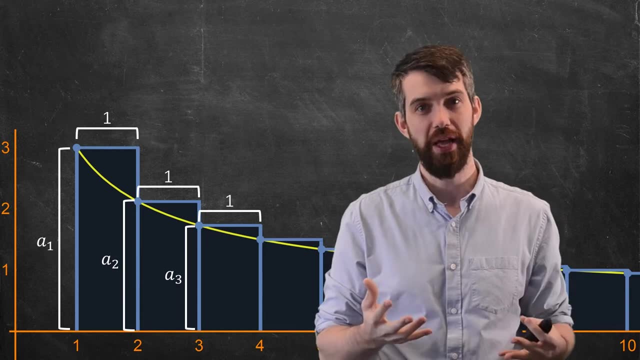 going to be a3,, a4, and so on down the line. So then, the area of the 1st rectangle is 1 times a1.. The area of the 2nd rectangle is 1 times a2.. And generally, if I want to talk, 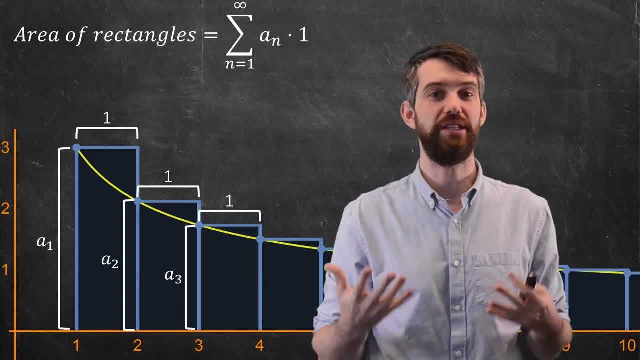 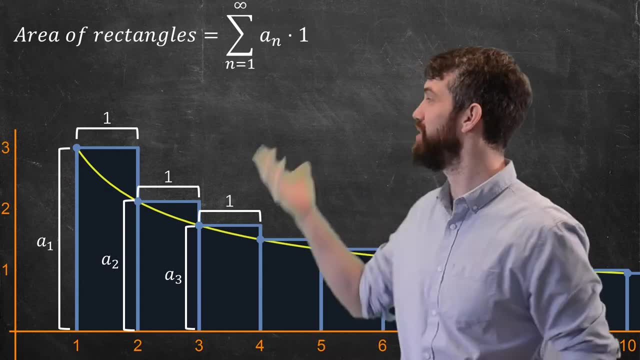 about the area of all of the rectangles. this is going to be a summation, a sum from 1 to infinity, of these heights, a1 times these widths, 1. Multiplying by 1 doesn't do anything, so I can get rid of that. So what I have is a geometric way. 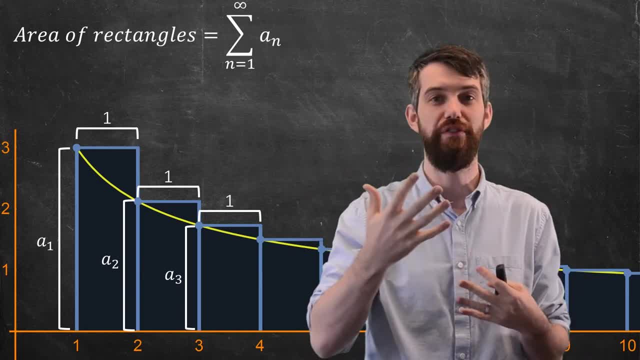 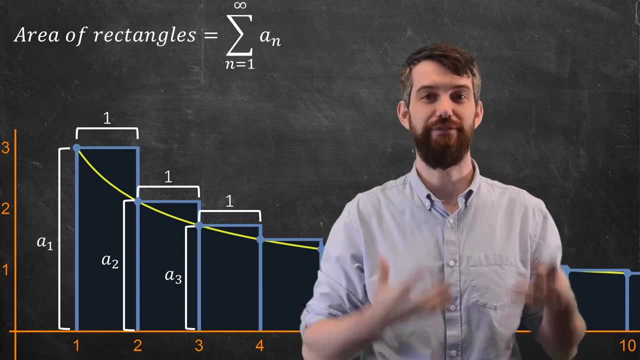 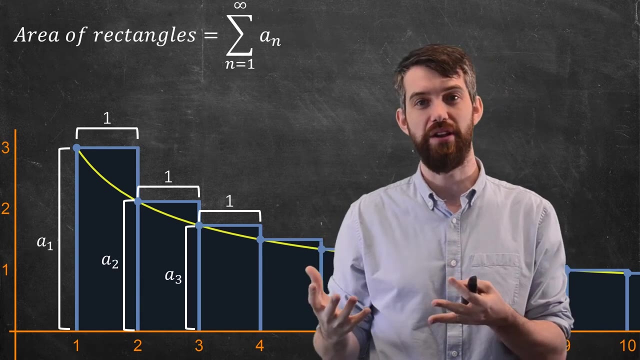 of thinking about what a series is. The summation from 1 to infinity, of a, n can be thought of as the sum of these particular rectangles. And because I have this function of the continuous real variable x, the yellow curve underlying it, I can relate the sum of these rectangles to the area under that curve. 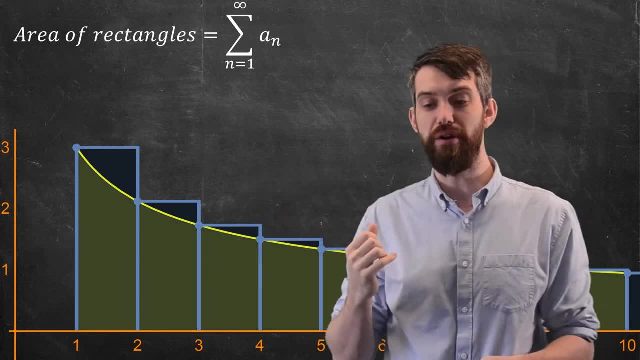 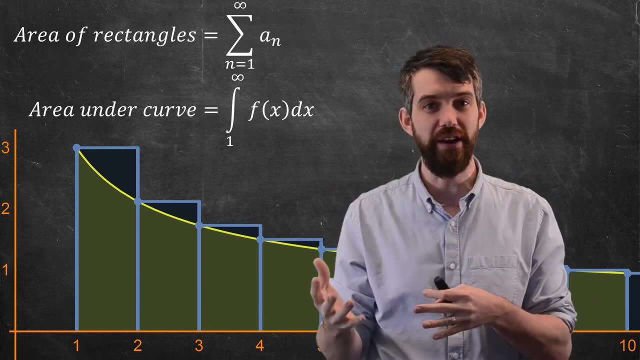 Indeed, if I get rid of all of this, the area under the curve is just shaded in here in yellow. It's in fact an integral. It's the integral from 1 up to infinity of f, dx. So there's actually two different geometric things going on here. 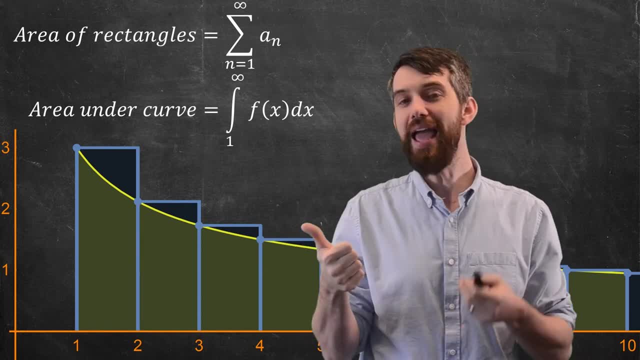 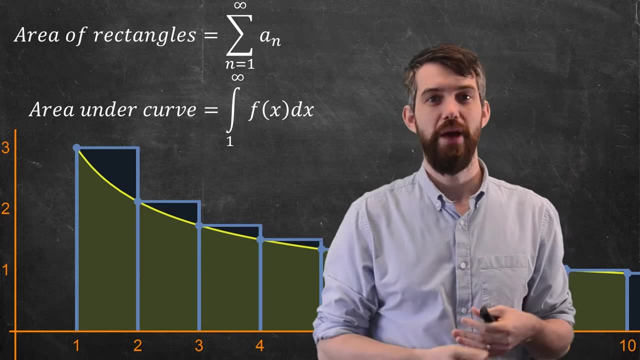 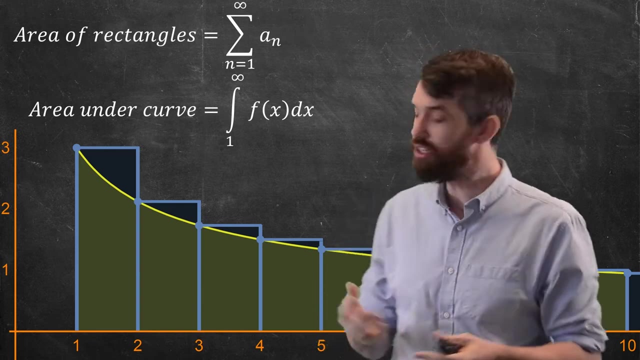 The improper integral, the integral from 1 up to infinity, of f, dx, and this infinite series which represents the sum of all these rectangles. Now if, in this specific example, my function is continuous, my function is decreasing and my function is positive, And in that scenario there's a relationship between: 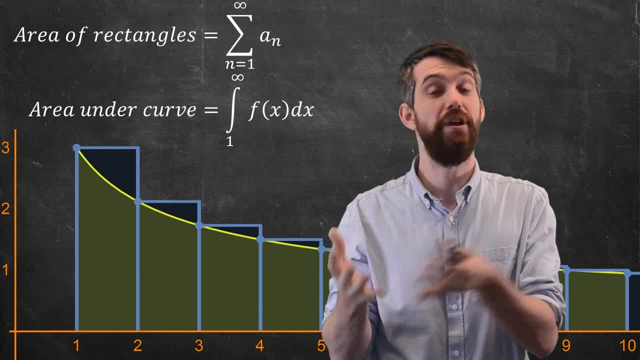 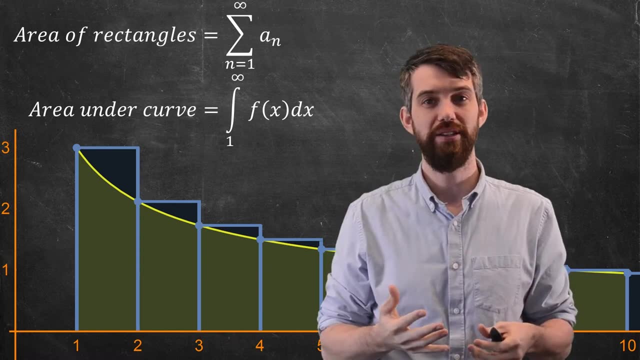 these two things. Notice how the rectangles are always bigger than the portion that comes from the area of the curve. There's little bits more sticking out in the area of the rectangles than the curve. So in this example what we have is a relationship. We say that the improper integral is 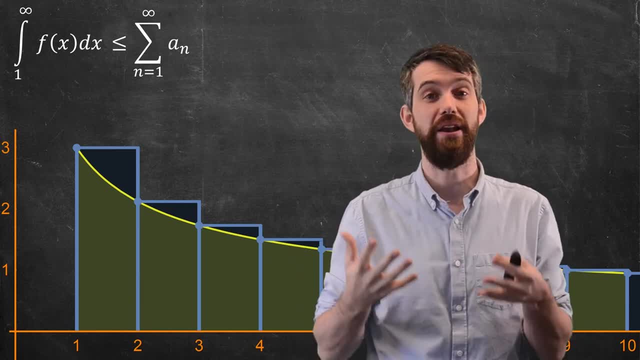 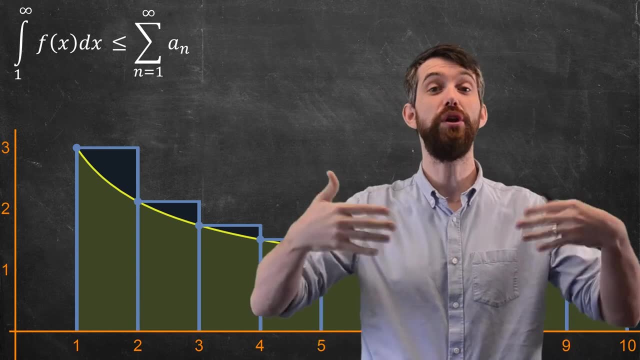 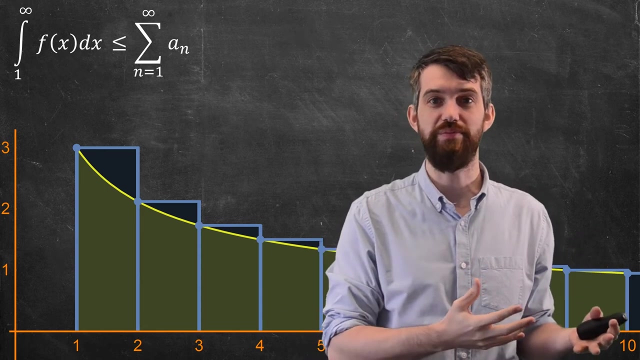 strictly less than the area of all the rectangles, strictly less than the series. Now, both of these things- I'm comparing the improper interval and the infinite series- both of them trundle off to infinity. They take either x going to infinity or n going to infinity. So the questions that we want to answer are: 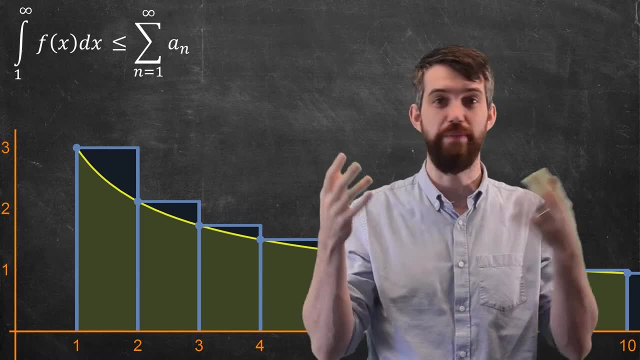 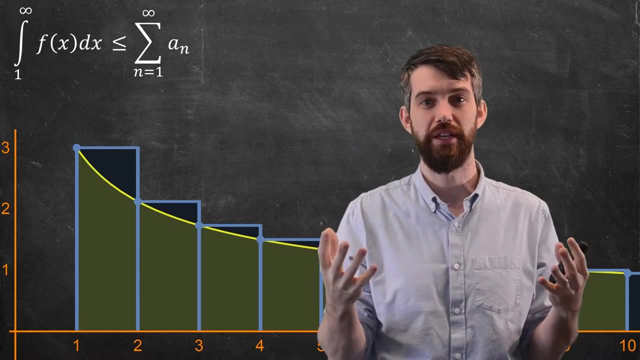 does this thing converge? does it diverge? they both converge, do they both diverge? does one convergent to the other? That's the kind of question we want to do when we're comparing these improper integrals to these infinite series, And 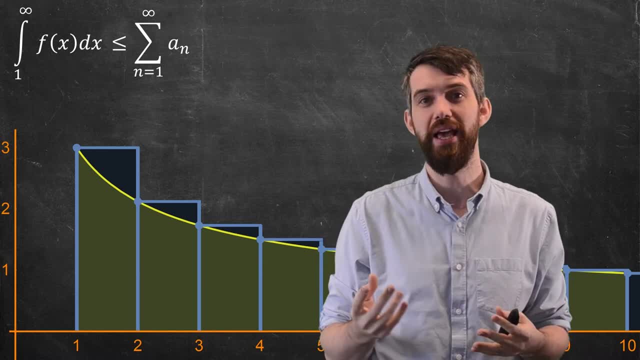 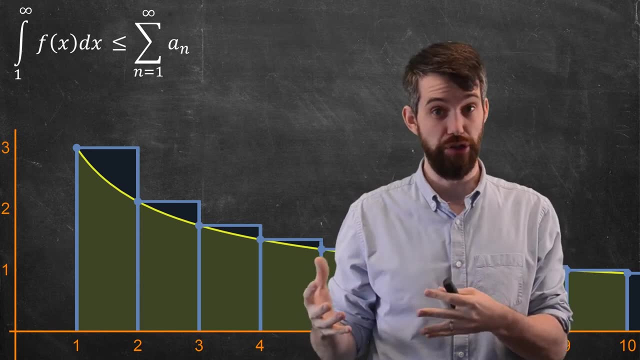 in this case, when there's this inequality between them, where you say that the improper integral is strictly less than the, you get the following fact: Imagine the improper integral diverged, the smaller one, so the area under the curve. Imagine that diversion went to infinity. Then the 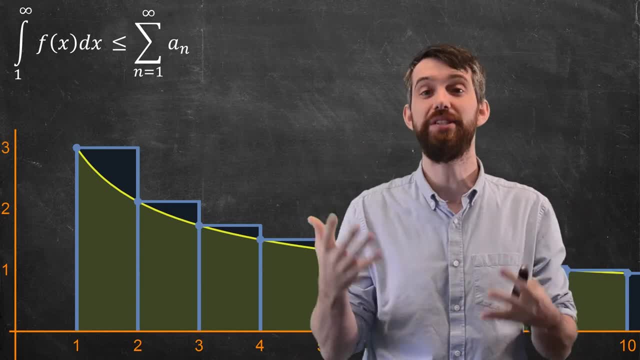 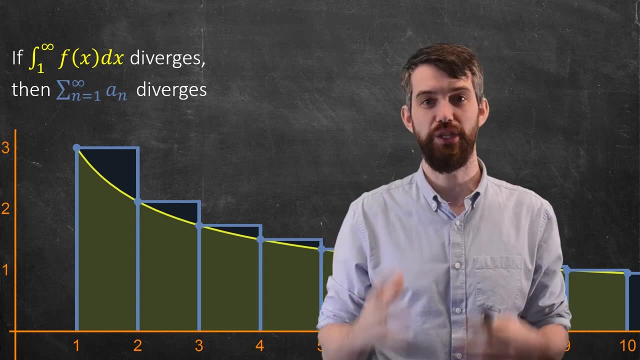 series, which, geometrically, is something that is bigger than that, must diverge as well. So in other words, I can say that if indeed the improper integral diverges, the series does as well, And this was true in that case where your function is. 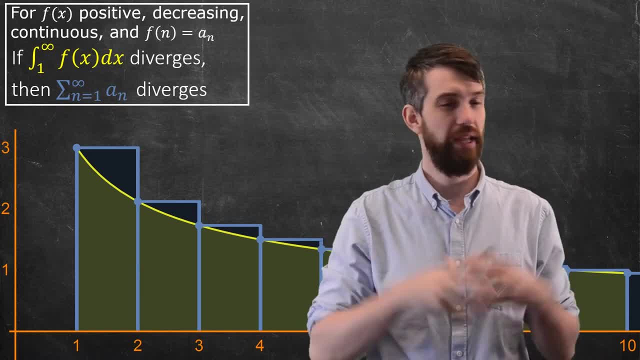 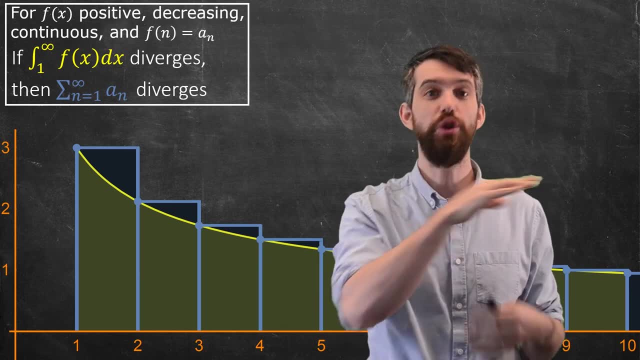 positive, it is continuous and it is decreasing. In fact, these assumptions are quite important. For example, if it was not going to be decreasing- like sometimes it went down and sometimes it went up, you wouldn't have that inequality that applied everywhere, where always the rectangles were bigger than 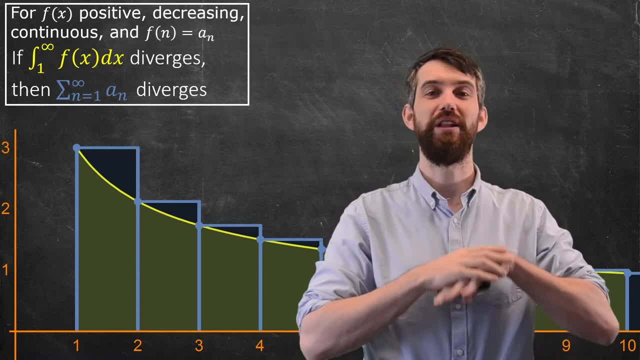 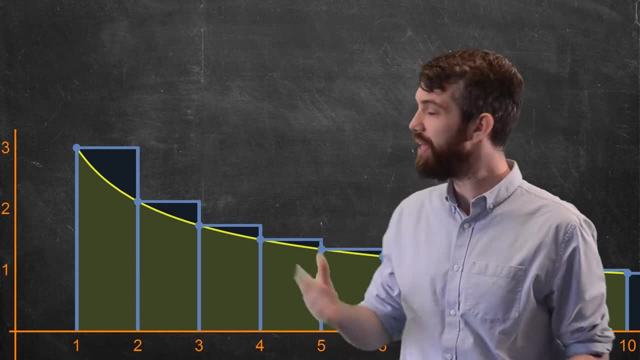 the corresponding version of the improper integral. Now, I've only really just done half of it. For example, let me do the other side, the other inequality. In the next example, I'm going to replace the left endpoints, which is what I have. 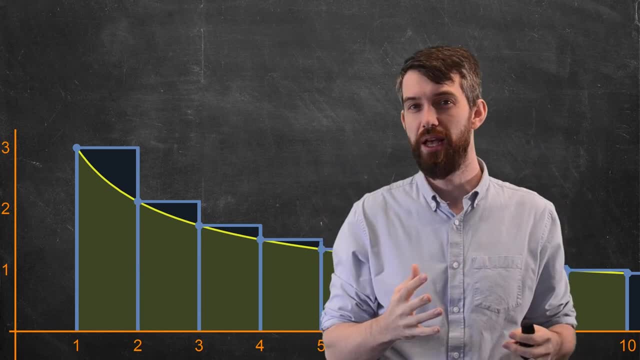 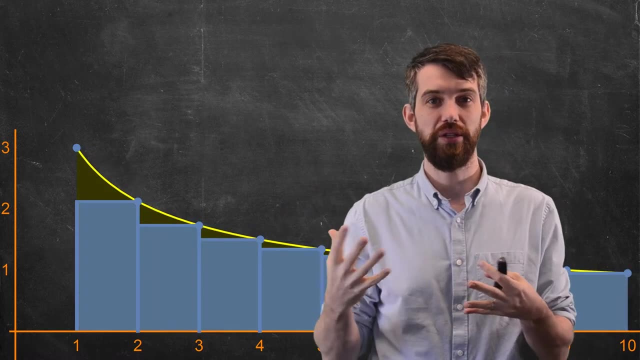 right now, All these rectangles represent left endpoints on each of the intervals, And instead I'm going to use right endpoints, So it looks instead like this: That is, all of my rectangles are smaller. Their widths are all the same. Their widths are all just going to be 1.. But now 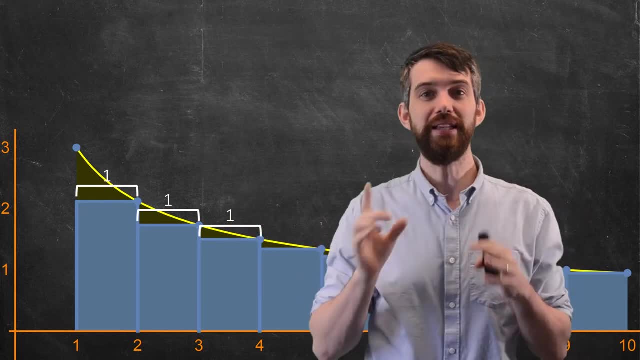 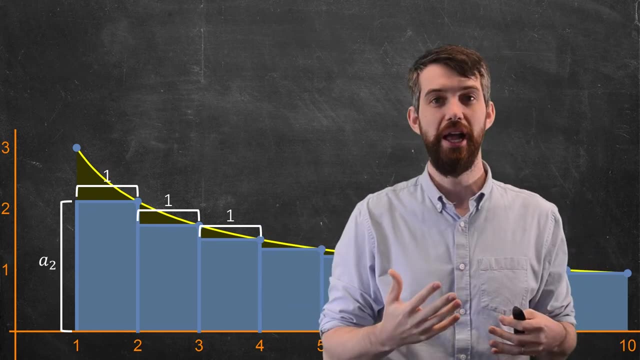 if I think about the leftmost, the first rectangle here, its height is not a 1,, it's a 2, because I'm using the right endpoint. So this, the first one, has this height of a 2.. The second one has a height of a 3.. The third one has a: 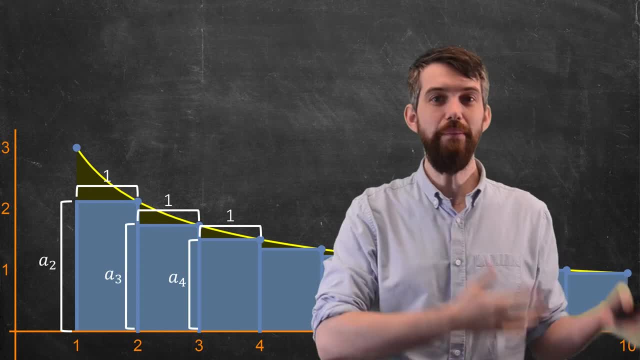 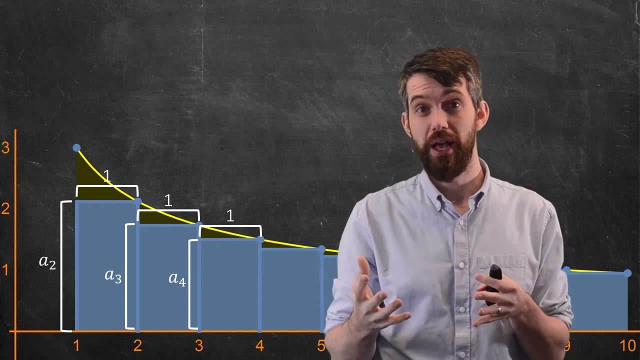 height of a 4, and so on. So I can make an inequality again, but it's a different one. That is to say, if I want to talk about the areas of the rectangles, I'm no longer starting at a 1.. I'm starting at a 2.. A 2 represents the 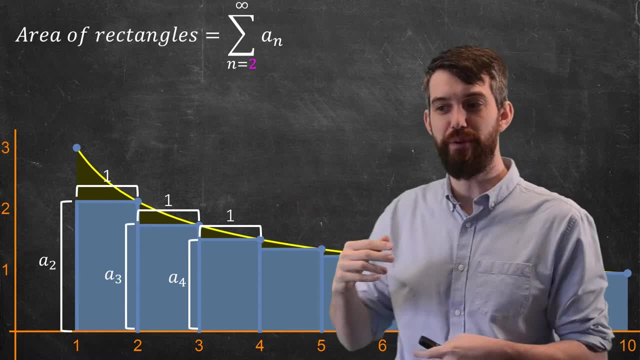 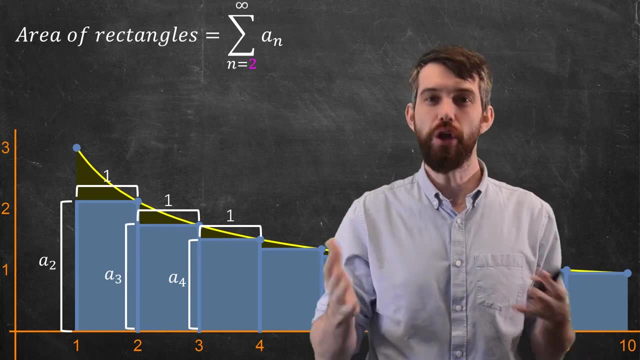 first rectangle. I look at it So it's not quite the same series before, not the sum from 1 to infinity, the sum from 2 to infinity, And you might think that's a big difference, but it really isn't. If I ask the question like, does a series? 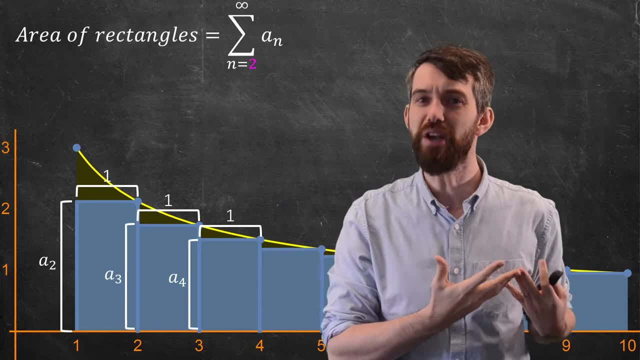 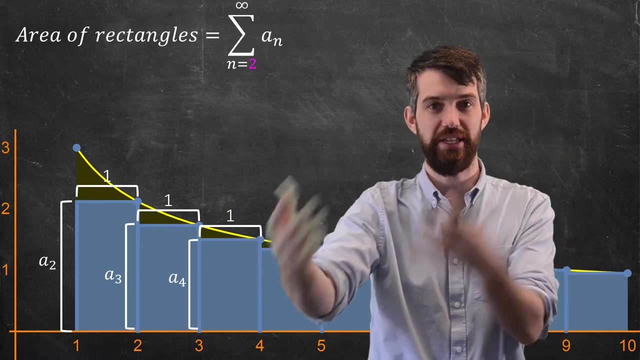 converge. What happens for the first term doesn't matter. Whether it converges is a question of: as you go off towards infinity, you add more and more and more things. Does that add up to a finite number? Does it diverge? But if I just change the value of the first 1, or heck the first? 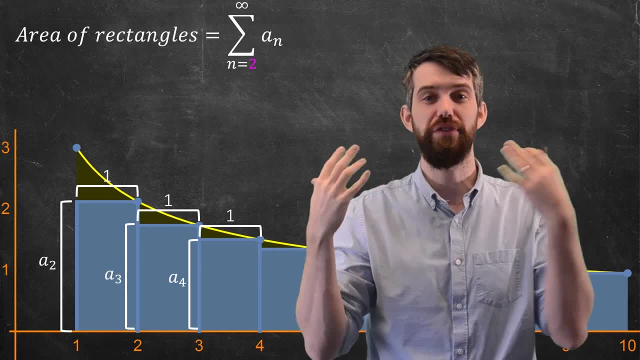 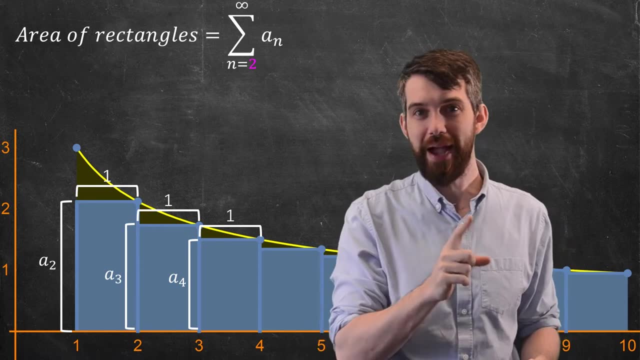 finite number of terms. it doesn't make a change to the question of convergence or divergence, So doing n equal to 1, n equal to 2, same difference. But it matters here from the perspective that I am going to contrast this with. indeed, 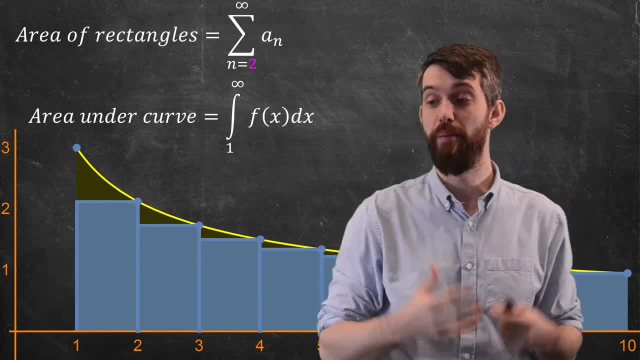 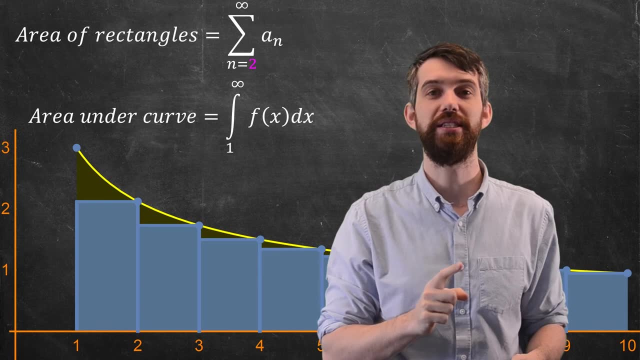 the improper integral from 1 up to infinity And for the improper integral from 1 up to infinity of f. that's the integral under the curve. Now my inequality is the other way around, which is to say that the improper integral is going. 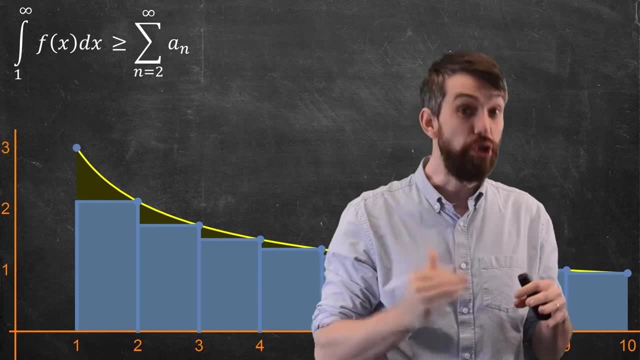 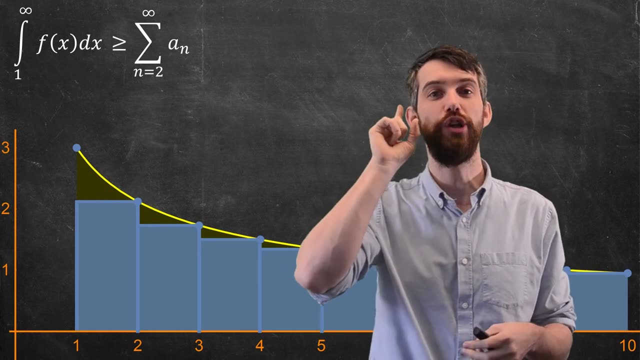 to be the bigger one. It is bigger than this series, from 2 all the way up to infinity. And so now, when I do my analysis, it goes the other way around. Imagine the improper integral not diverges. Imagine it converges, So the improper integral is converging. Well, 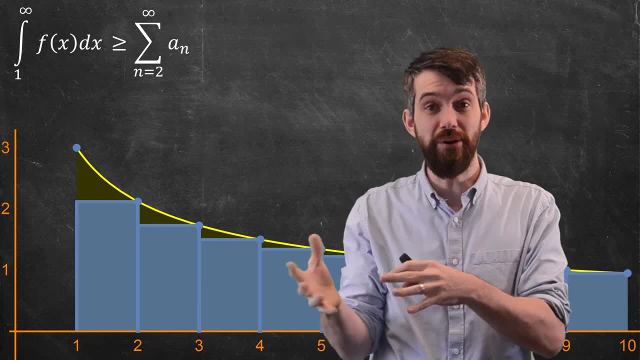 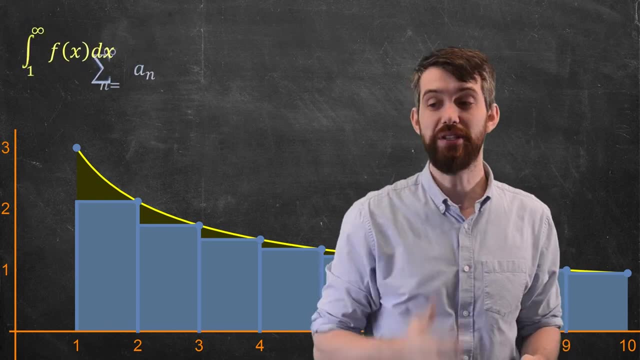 in that scenario that tells me that it is bigger than the series. So if the bigger thing converges, the smaller thing, the series, must converge as well. So I get the other side of my theorem. It says that if the improper integral converges. 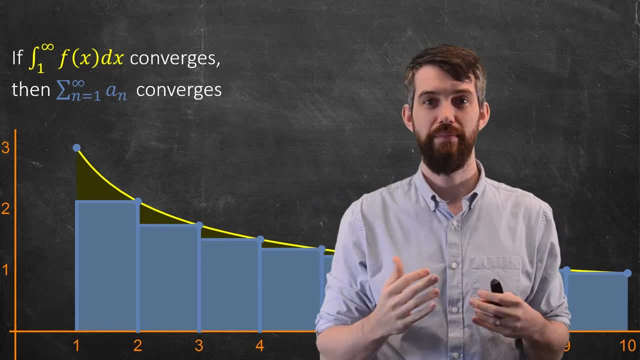 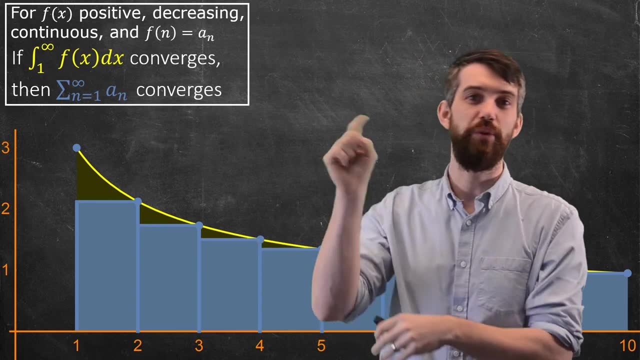 then so too, indeed, does the series. And again, this is under the context of a function which is positive and decreasing and continuous, where the function values. when you plug in the n, just give your series terms. Those are my assumptions. So I really have two parts.